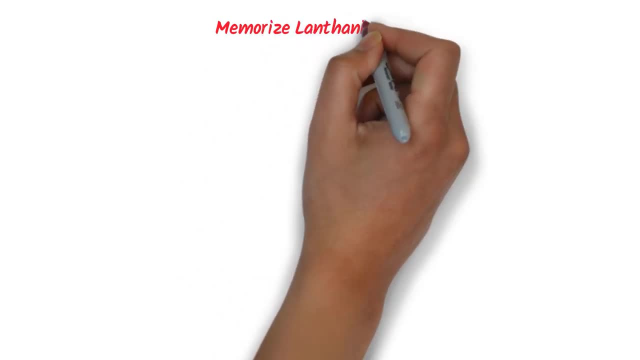 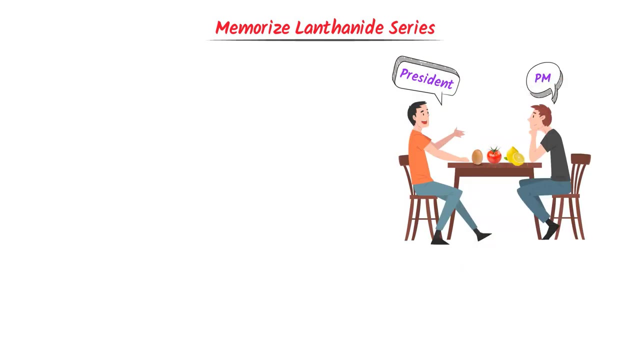 Firstly, let me teach you my personal trick to memorize lanthanide series. For example, consider the President and Prime Minister of Canada sitting at the table. I say Canadian President and Prime Minister at same European golden table. Secondly, on the table there are eggs, tomato and lemon. 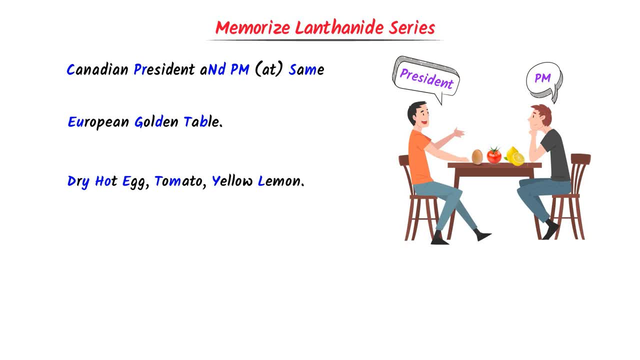 I say dry hot egg, tomato yellow lemon. So I say Canadian President and PM at same European golden table: dry hot egg, tomato yellow lemon. We know that lanthanide series starts from lanthanide. I write lanthanum L-A. 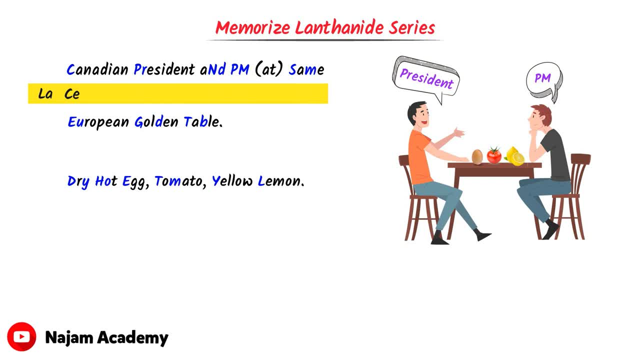 Now the C in Canadian stands for C-E. P-R in the President stands for P-R. N-D in the And stands for N-D. P-M stands for P-M. S-M in the Same stands for S-M. E-U stands for E-U. 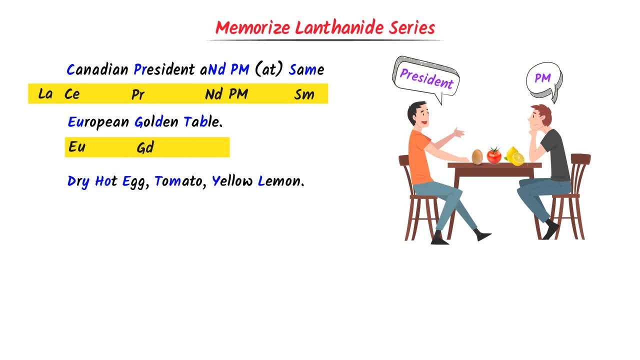 G-N-D in the Golden stands for G-D. T-B in the Table stands for T-B. D-Y in the Dry stands for D-Y. H-O in the Hot stands for H-O. E in the Egg stands for E-R. T-M in the Tomato stands for T-M. 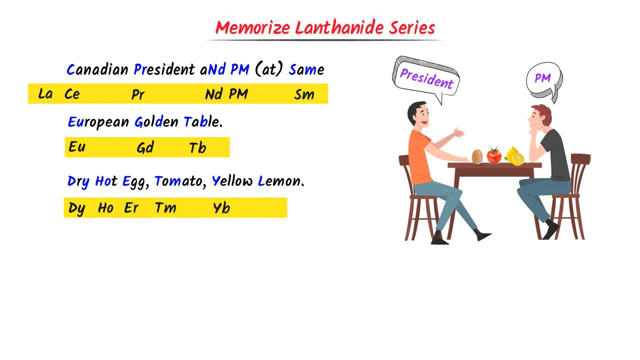 Y in the Yellow stands for Y-B, L in the Lemon stands for L-U. This is the lanthanide series. I challenge you that you will not find this mnemonic in any book or in any video. Just remember this picture of Canadian President and Prime Minister. 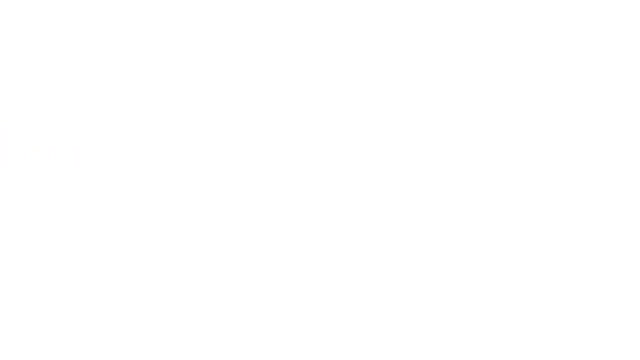 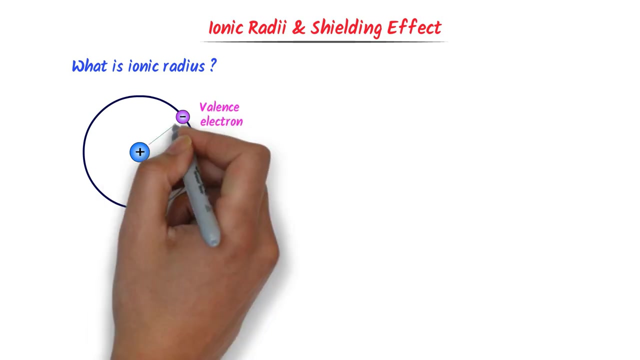 Now, to learn lanthanide contraction, we must learn the concept of ionic radii and shielding effects. For instance, what is ionic radius? Well, consider this atom. We know that this is a valence electron. Let the distance between the nucleus and the valence electron is r. 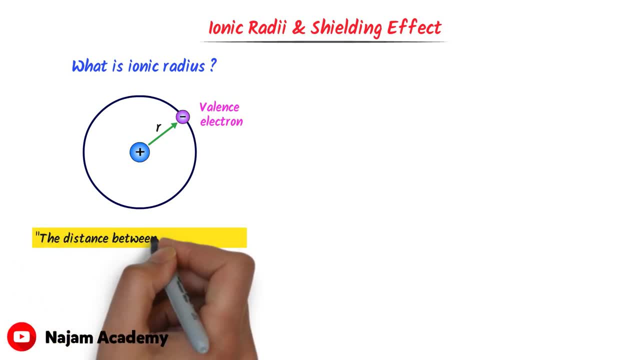 We define ionic radius as the distance between valence electron and the nucleus is called ionic radius. Let me repeat it: The distance between valence electron and the nucleus is called ionic radius. Hence this r represents ionic radius. Now, what is shielding effect? 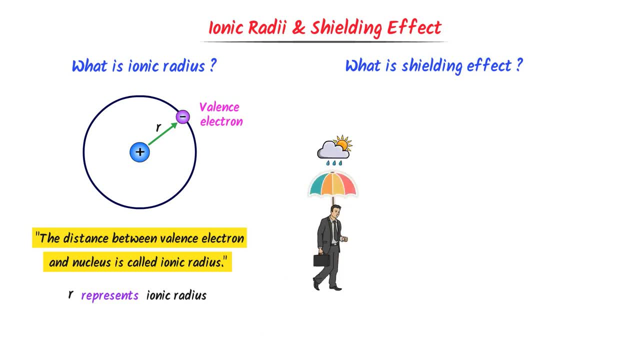 Well, consider this man holding this umbrella in the rain. We know that this umbrella protects or shields this man from the rain. Or we say, this man doesn't receive any raindrops. Similarly, consider this atom, The electrons, in the third shell shield. 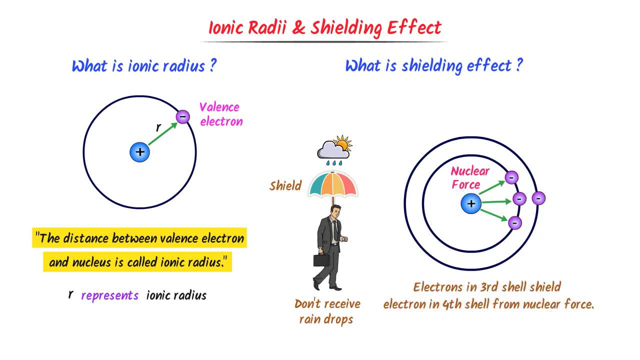 the nuclear force on the electron and the fourth shell. Let me repeat it: The electrons in the third shell shields the nuclear force on electron and the fourth shell. We say that the electrons in the third shell act like umbrella, which decreases the nuclear force on outermost electron. 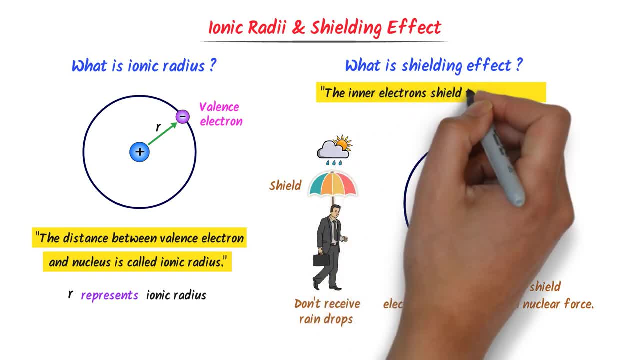 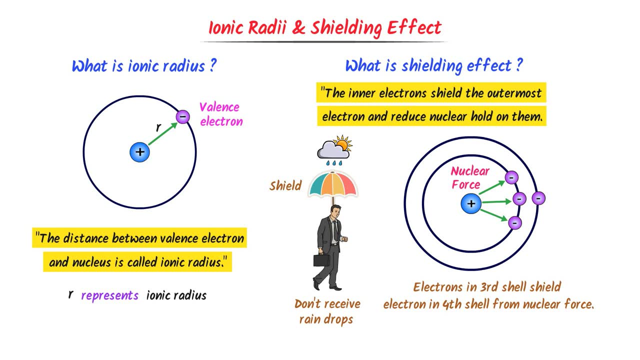 Hence we define shielding effect as the inner electrons shield the outermost electrons from the nuclear force and reduce nuclear hold on them. This effect is called shielding effect. Let me repeat it: The inner electrons shield the outermost electrons from the nuclear force and reduce nuclear hold on them. 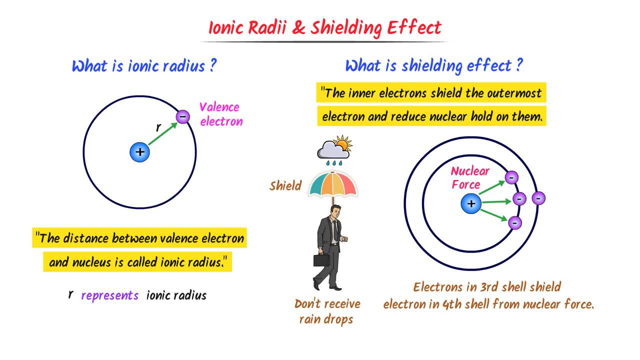 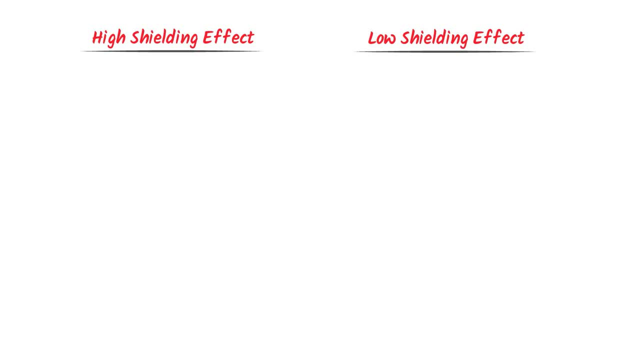 This effect is called shielding effect. Now let me teach you the concept of high shielding effect and low shielding effect. In case of high shielding effect, consider this atom. Let this orbital strongly block or shield the nuclear force. Now the electron and this orbital receive less nuclear force. 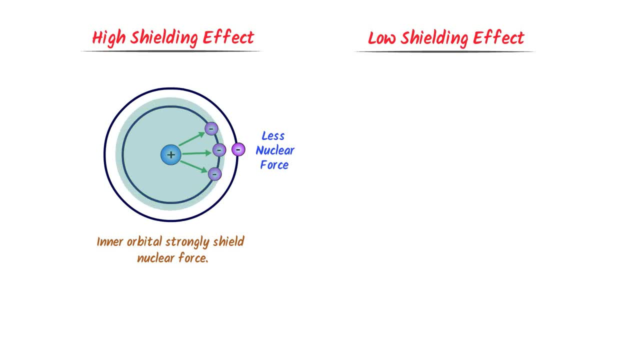 As a result of this, it will move an outward direction and the ionic radius or size of an atom increases. On the other hand, consider this atom, Let this orbital partially block or shield the nuclear force. Now the electron and this orbital receive more nuclear force. 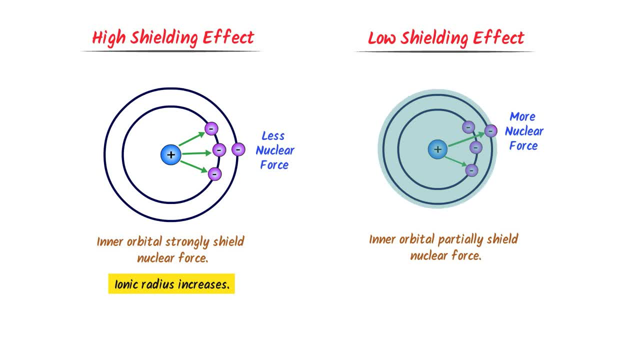 As a result of this, it will move in inward direction and the ionic radius or size of an atom decreases. Just note it down that the high the shielding effect, the larger is the atomic size or ionic radii, While the less is the shielding effect, the smaller is the atomic size or ionic radii. 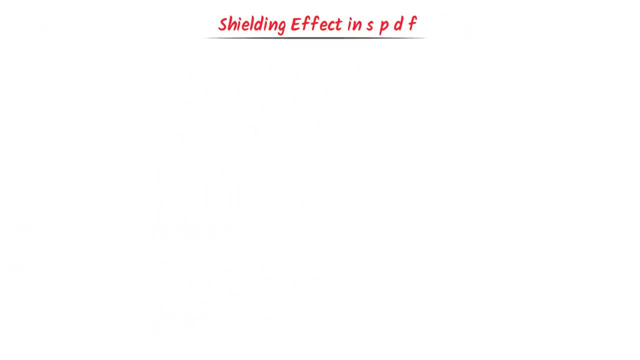 Lastly, let me teach you shielding effect and spdf orbitals. The order of shielding effect is like this: S orbital has highest shielding effect, while F orbital has lowest shielding effect. But I do not teach this concept. I teach you my own concept. 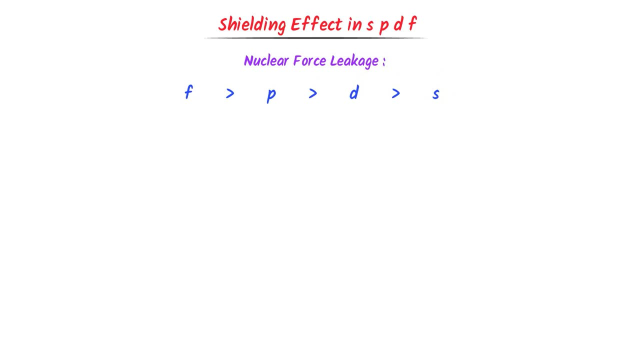 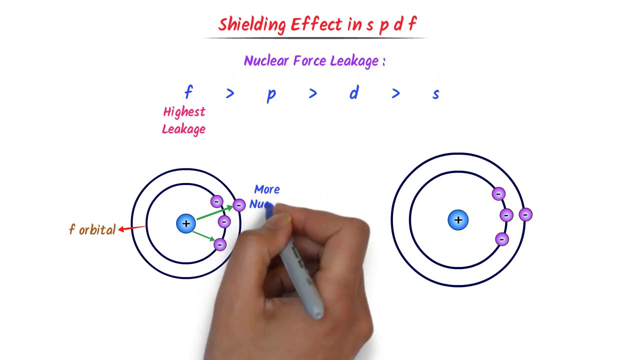 I say, the order of nuclear force leakage is like this, For example. consider these two cases. In the first case, this is F orbital. According to this order, the nuclear force leakage of F orbital is maximum. Hence nuclear force will leak from F orbital and this electron will receive strong pull. 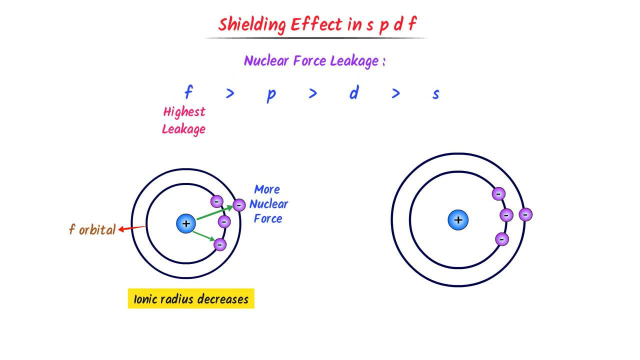 As a result, the atomic radius decreases. Thus we say that the more the nuclear force leakage, the smaller is the ionic radius. In the second case this is S orbital. According to this order, the nuclear force leakage of S orbital is minimum. 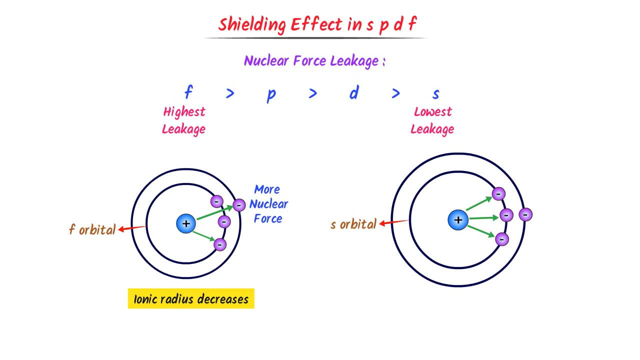 Hence no nuclear force leaks from S orbital, and this electron receives negligible amount of nuclear force As a result, this atomic radius increases. Thus we say that the less the nuclear force leakage, the more is atomic radius or atomic size. If you have learnt all these important concepts, 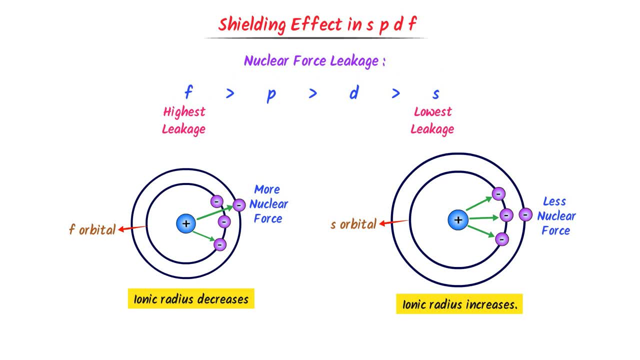 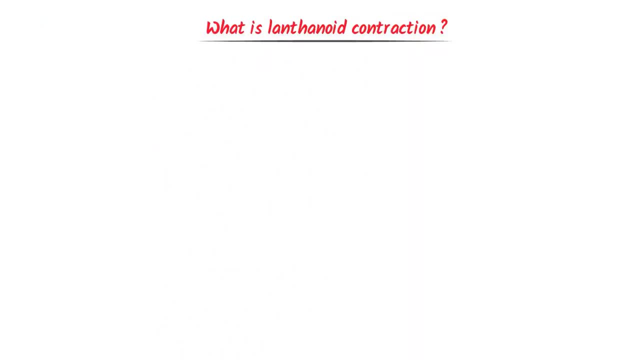 I hope you have learned something. I hope you have learned something. I congratulate you. You have already learnt the concept of lanthanide contraction. Now, what is lanthanide contraction? Well, consider this lanthanide series. We know that lanthanum is the first element and Lu is the last element. 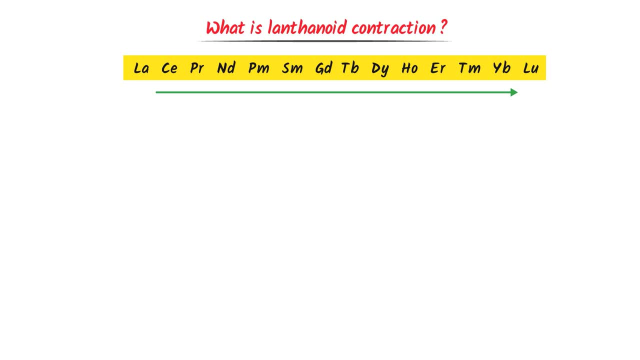 Now listen carefully. If we go from left to right, the atomic radius of lanthanum series decreases from 187 pm to 172 pm. Let me repeat it: if we go from left to right, the atomic radius of lanthanum series decreases. 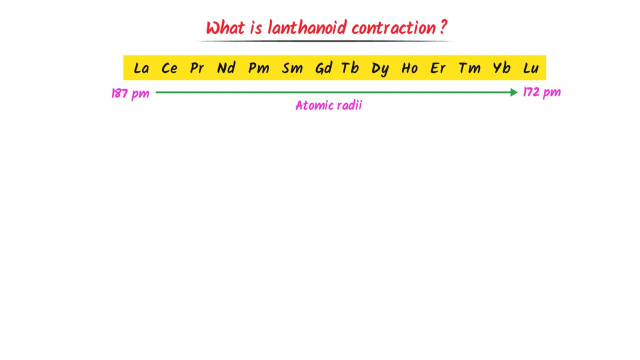 from 187 pm to 172 pm. This decrease in atomic radius of lanthanum series is called lanthanide contraction. The most important question is: what causes lanthanide contraction? The answer is simple. Consider this atom of lanthanide series.